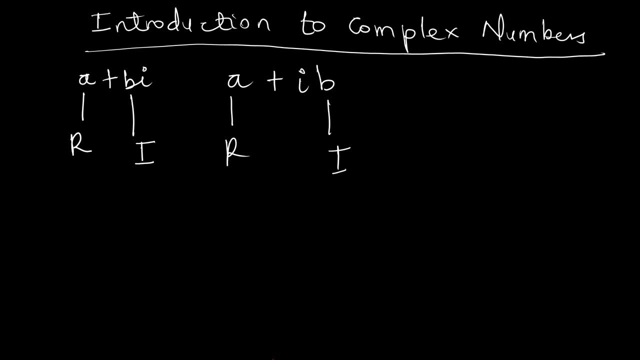 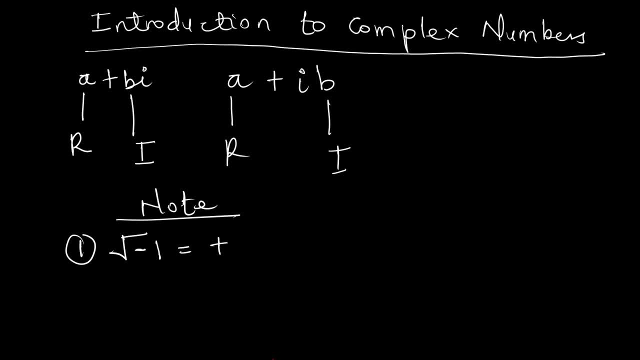 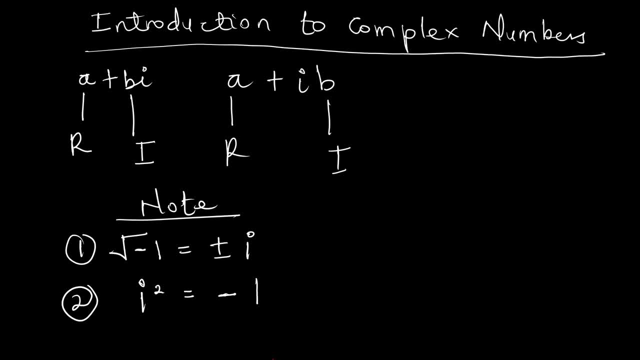 4. 4. 4.. So these two are the assumptions of what you have to know in the course of complex numbers. Alright, but one may ask: why is it that square root of negative 1 doesn't represent matters? is plus or minus i and y is i, squared is equal to negative one. i shouldn't forget that the set 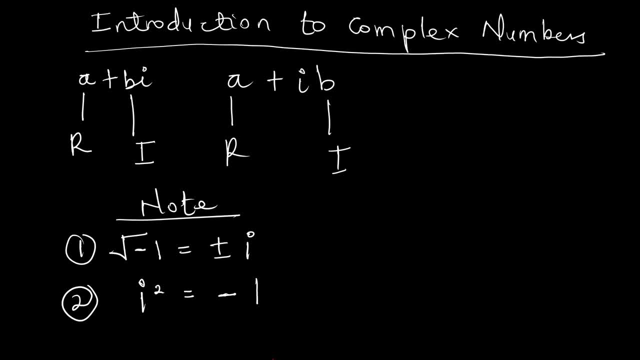 of real numbers will not allow us, or not allow solution to all quadratic equation, right. for example, when we have s squared plus one is equal to zero, it's going to imply that s squared is equal to negative one, right, but negative one s squared is equal to negative. one has no real solution. 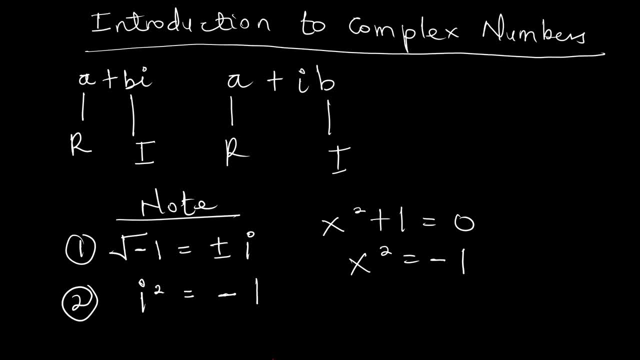 since s squared is always positive for your numbers. normally you have s squared minus one is equal to zero then. yet at the end of the day you are going to have s squared is equal to at one. so, more times, or mostly, s squared is always positive for your numbers. however, we can 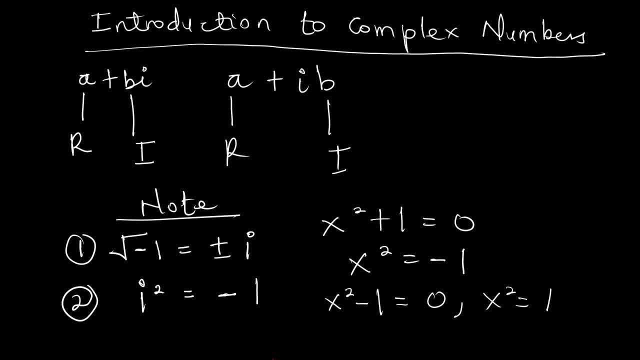 do that in the next lesson. Thank you, come the difficulty. by enlarging the set of real numbers to include a new number denoted i, with the property that i squared is equal to what negative one. so here the bottom line is that the i introduction of i squared is helping us to solve. 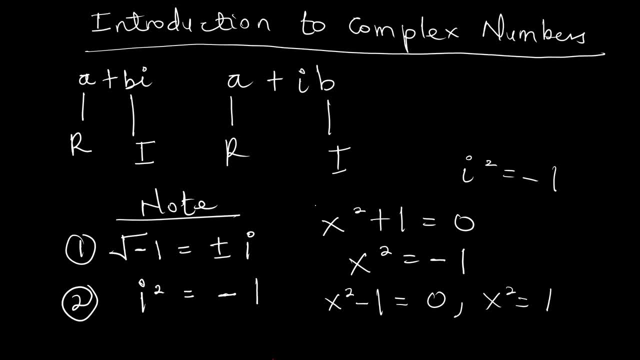 complicated equations or complicated quadratic equations in this form, right? okay, now let's look at this part. okay now, the introduction of this new number. i help us to overcome the problem of finding the square root of a negative number, like i i used or explained earlier. if we have s squared. 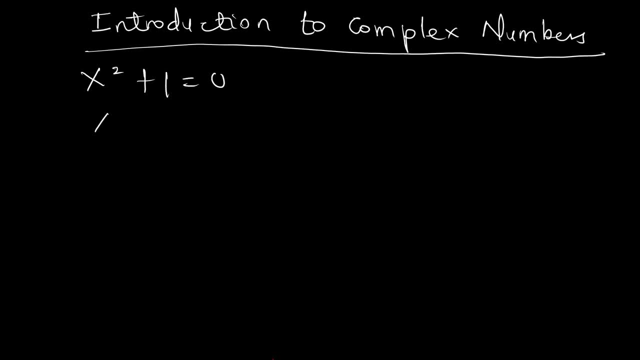 plus one is equal to zero. we are going to have x. squared is equal to negative one and x will be equal to square root of what negative one, or plus or minus square root of negative one. when you you punch square root of negative one on the calculator, you're going to 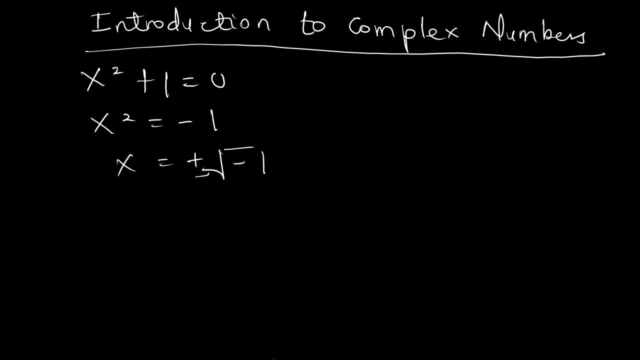 guess math error? it's not going to be possible, but the introduction of complex numbers will help us to solve equations like this. so let's try solving one or two examples. let's take the square root of negative 25. what would be the answer, square root of negative 25, when you punch this on the? 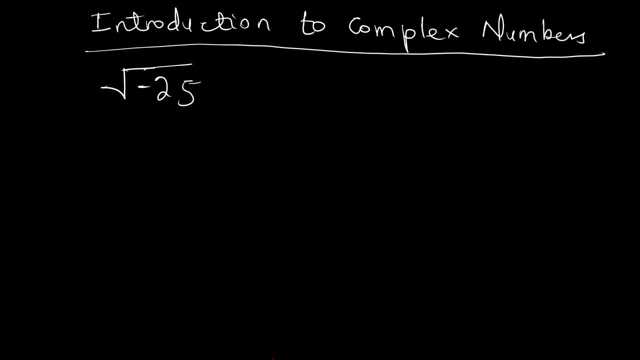 calculator, you are going to get math error, but the introduction of complex number has made this possible. okay, so let's start. so square root of negative 25 can be written as negative. negative 1 times 25 right plus negative 1 times 25. negative 25 is the same thing. 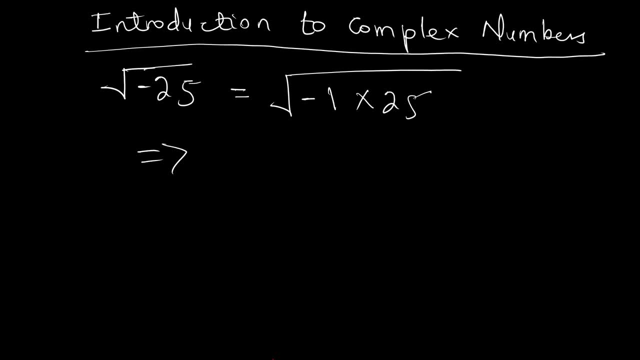 then a property of set. when we have two numbers multiplying under a square root, you can separate the two numbers and give them their individual square roots, right? so you can say that here you have negative square root of negative one multiplying square root of what- 25. okay, 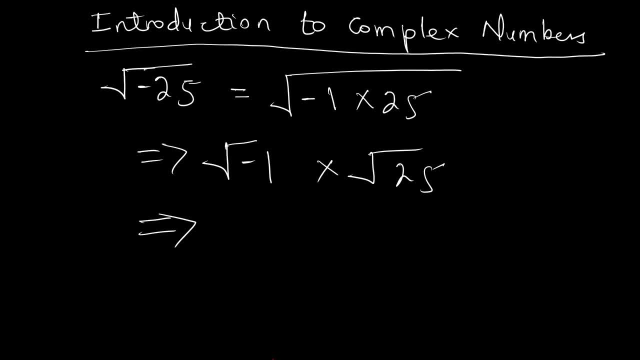 now, you didn't forget that. you just made mention of the fact that in complex numbers we always assume that square root of negative 1 is equal to what i, so we are using that property here. so if square root of negative 1 is i, then we are going to have i times what is square root. 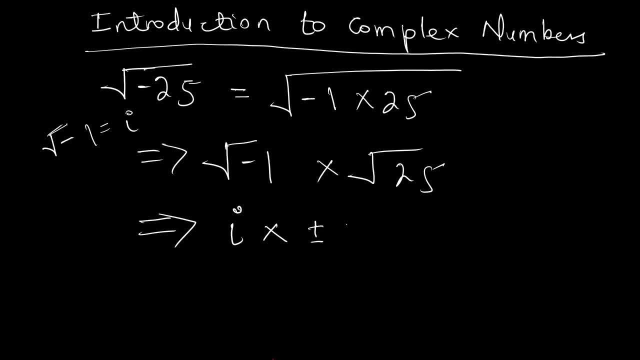 of 25, you will get plus or minus. what five, right? so here we have i times plus or minus 5. so you're going to give us plus or minus 5 i. so that is what you get when you find the square root of negative 25. when you take the square root of negative 20. 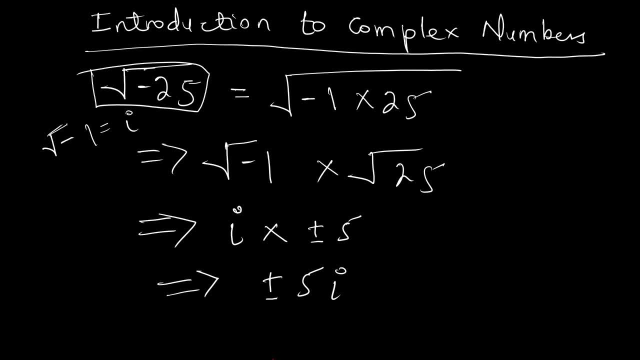 like you're going to get plus or minus 5, i okay. now let's take another example. okay, let's solve this quadratic equation: x squared minus 6, x plus 25. okay, previously, when you are solving quadratic equation and you have a discriminant which is: 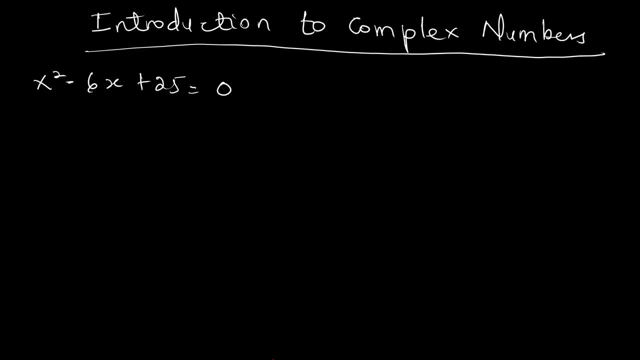 less than 0. the calculator will give you a complex number or it will tell you that there is no solution or has no real roots. right, okay. but the introduction of complex numbers has made this possible. we can solve this with the idea of complex numbers, so let's compare this to the general. 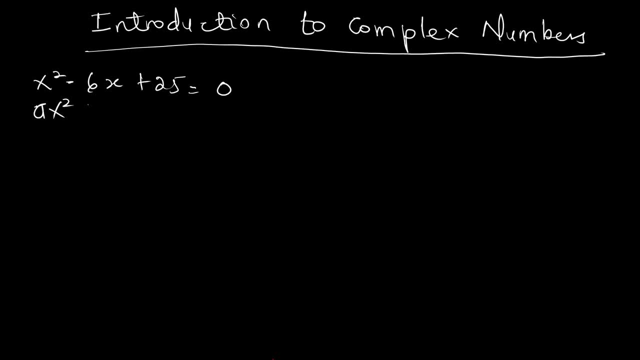 form of quadratic equation. so we are going to have a squared plus bx plus c equals zero, where a is equal to one because the coefficient of x squared is one, e equal to negative six and c equals 25.. then let's go to the quadratic formula. x is negative. 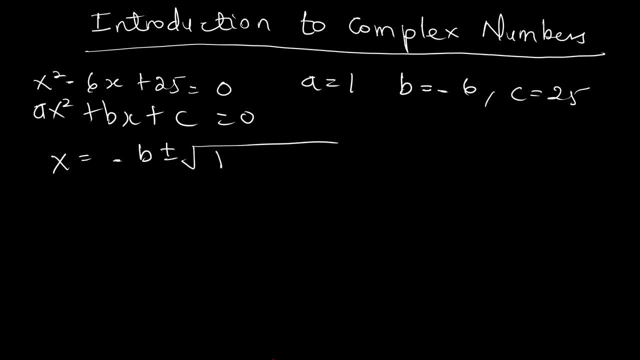 b plus or minus square root of e squared minus 4 is all over 2 a. let's do a substitution: negative b, so negative e, which is negative 6 plus or minus square root of e squared is negative 6 squared minus 4 a, which is 1 times c, 25, all over 2 a. sorry. 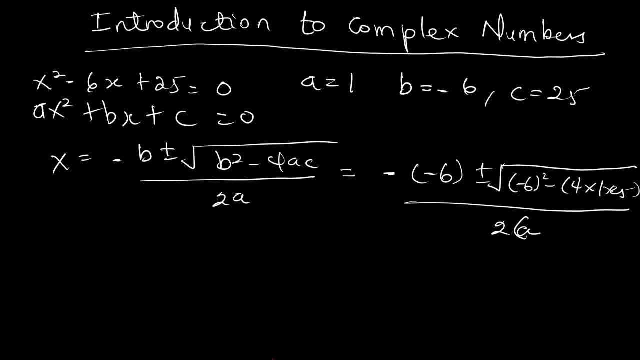 just multiplying one, two, two times one. all right now we are going to have: from here we're going to have positive six plus or minus square root of b squared negative c is all squared going to give us 36 minus 4 times 1 times 25 will give us 100. all over 2 a, which is two times. so how many pieces? 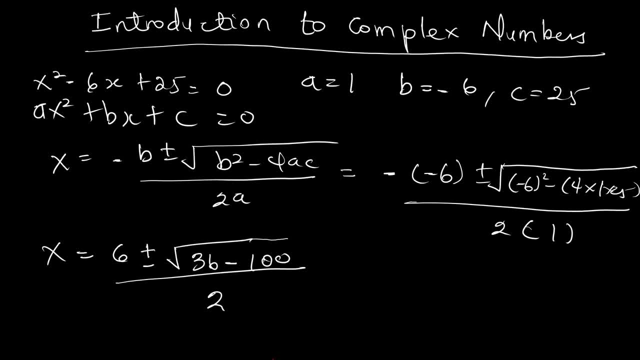 two. all right, let's simplify further. let me make space for this. it's quite simple. i just apply in there. okay, so we all look at all our favorite equations and we use this solution so i can represent the idea of complex numbers to solve quadratic equations which are having a discriminant less than zero. all right, 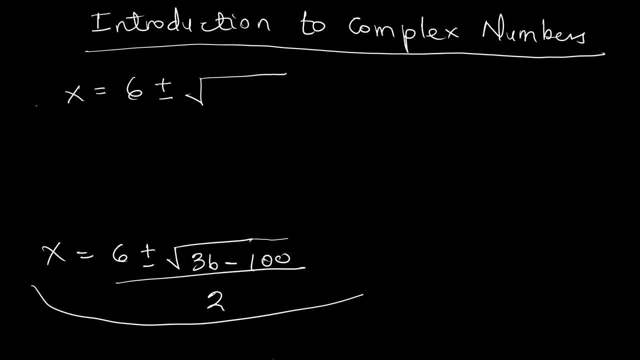 so from here we are going to have x equals six plus or minus. for other, 36 minus under is going to give us negative 64. so negative 64 all over 2, all right. so this implies that 6 plus or minus, X equals 6 plus or minus. we have square root of negative. 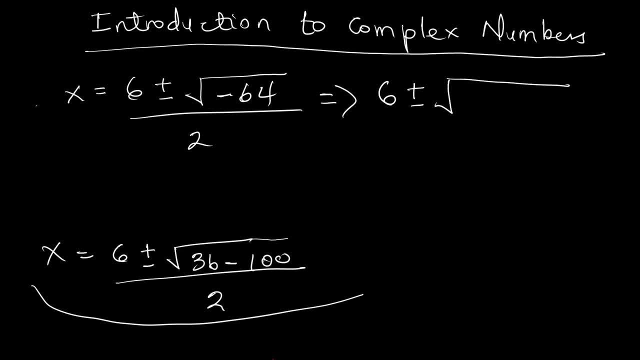 64. you, my, you can rewrite this as square root of 64 times negative 1, all about it. we are going to have six plus or minus square root of 64 times square root of negative 1. all right, we're wind yet. six plus plus. 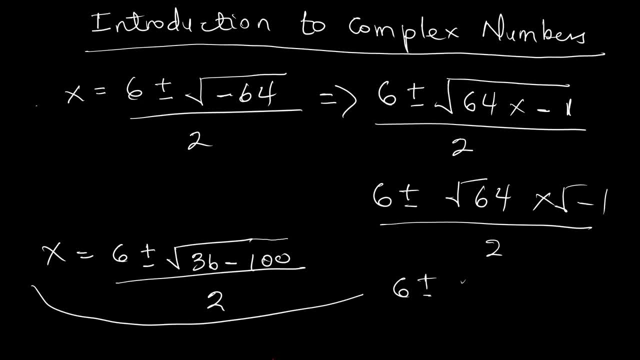 plus or minus. square root of 64 is what You know. that square root of 64, it says 8.. So 8 multiplying we have square root of negative 1. here We use our property that we know. So it would be what. 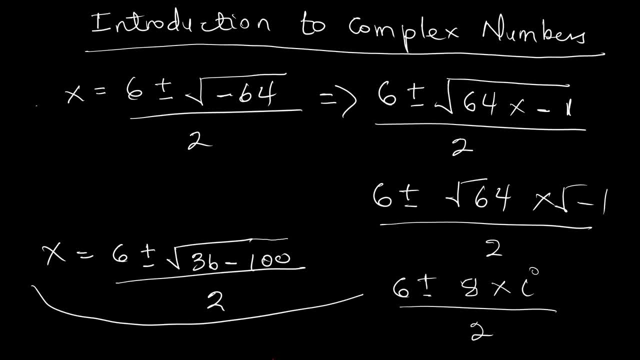 i all over 2.. Square root of negative 1 is i. We have 6 plus or minus 8 times i all over 2.. Let's continue. We are going to get 6 plus or minus 8i, because 8 is multiplying i all over 2.. 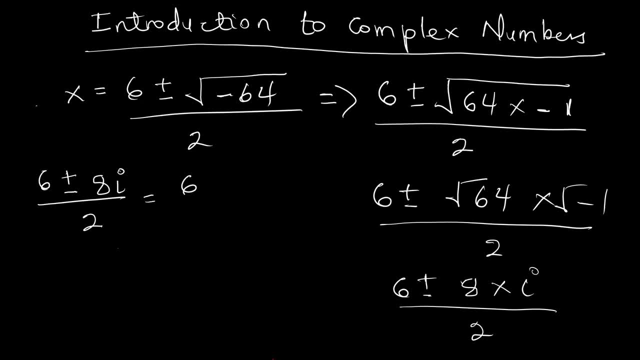 So sum of fraction 6 divided by 6 plus or 6 over 2 plus or minus 8i over 2. 6. We are going to give us 3 plus or minus 4i Splitting this. 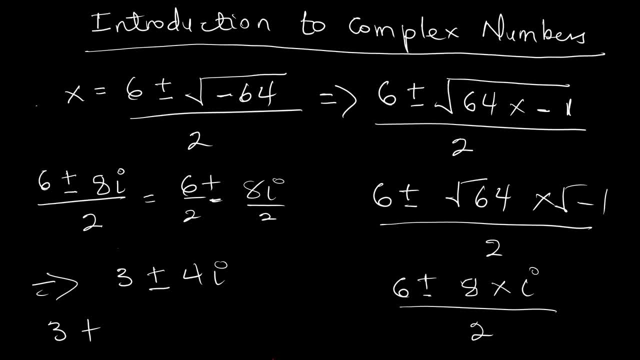 you can get two answers for x, as 3 plus 4i and 3 minus 4i. So this is how we use the idea of complex numbers to solve quadratic equations. That has a discriminant less than 0. And the discriminant is: 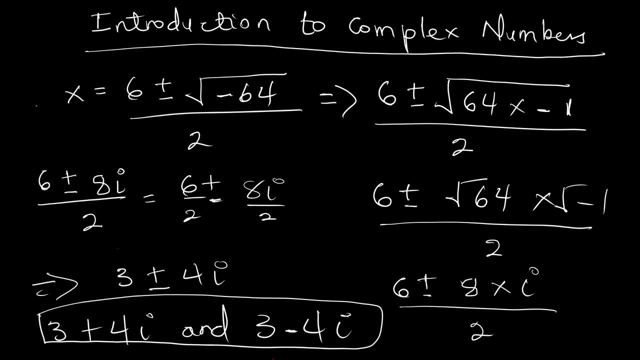 the b squared minus 4a's. So when you substitute your values and the b squared minus 4a's, the value of b squared minus 4a's is less than 0. That is negative. Then complex numbers is going to be 100.. 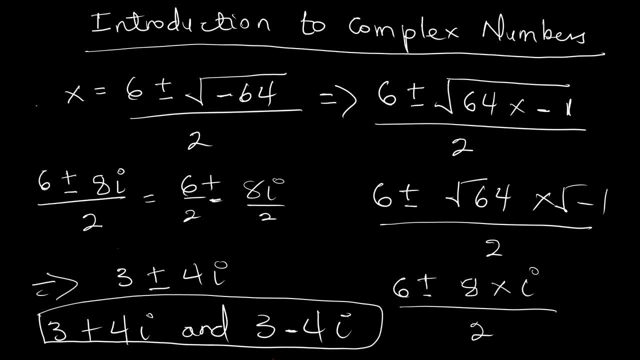 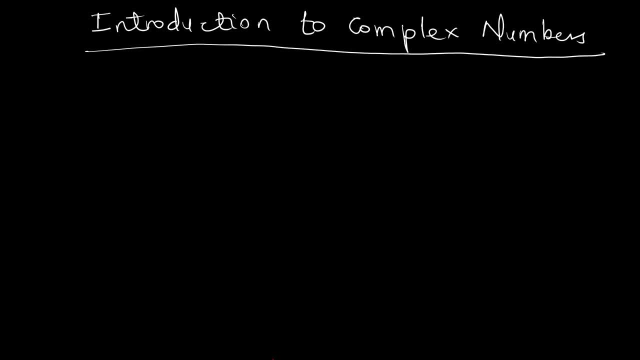 We are going to use complex numbers. Alright, Now let's move to the next thing Now. sometimes complex numbers are defined in terms of ordered pairs. What do I mean by that? Let's say a complex number denoted by z. We have a complex number denoted by z. 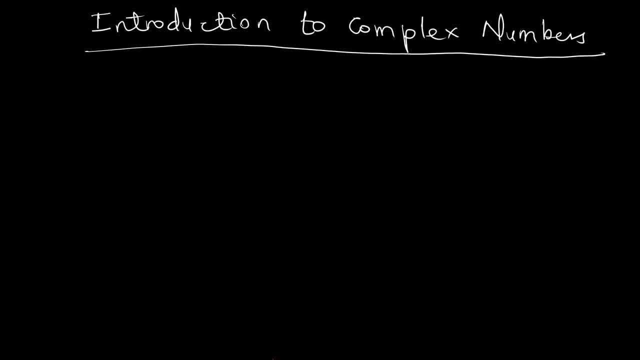 A complex number denoted by z can be defined in terms of an ordered pair, as z is equal to x comma y, This is the same as z being equal to x plus i, y or x plus y i, So the x here represents the real part. 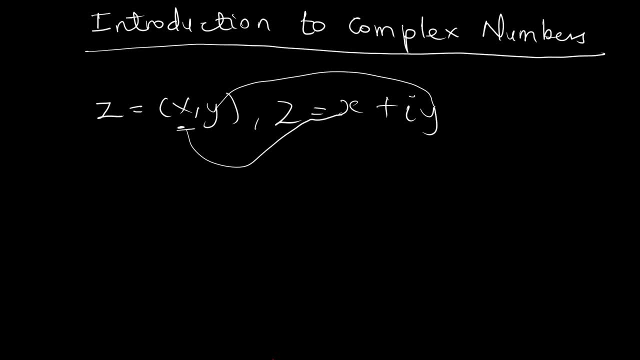 the complex number and the y represents the imaginary part. So in the ordered pair, the x part or the first part represents the real part, The second part represents the imaginary part. That's how sometimes you express complex numbers. 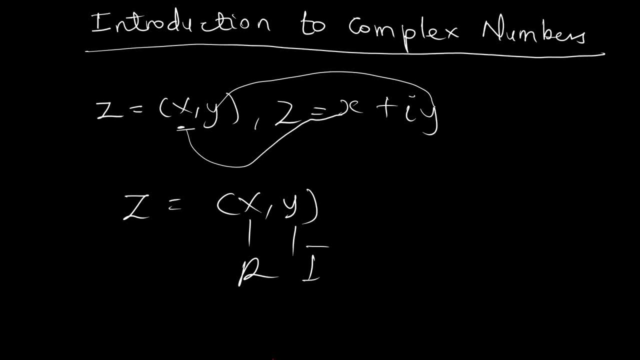 You express them as what? As ordered pairs? Now, let's move on to the equality of complex numbers. Now, let's move on to the equality of complex numbers. Now, let's move on to the equality of complex numbers As simple as ABC.